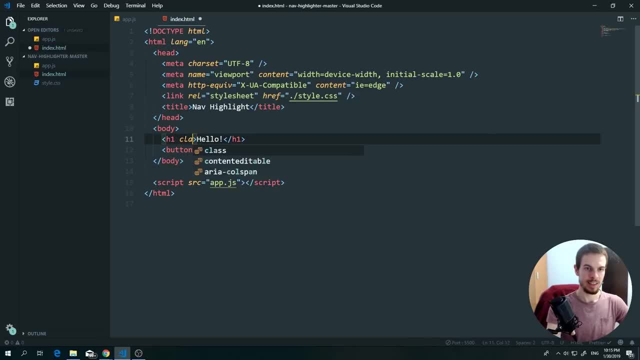 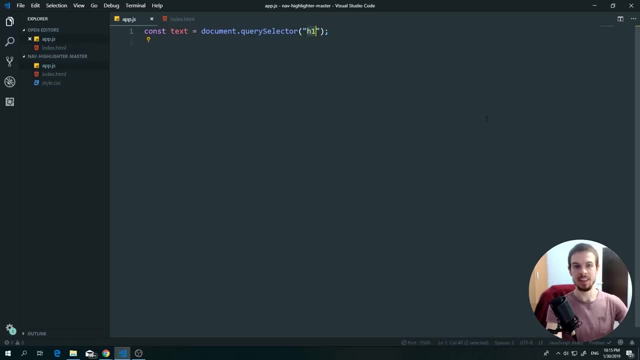 it like this: you're probably going to have a class on this, So we're going to add a class of title to this. So the way we can access these specific class is the same way we can do it in CSS, So by writing. 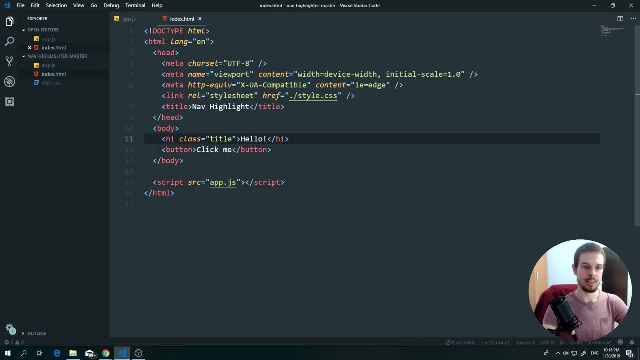 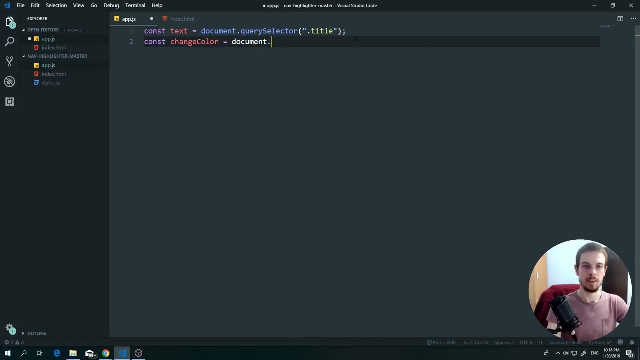 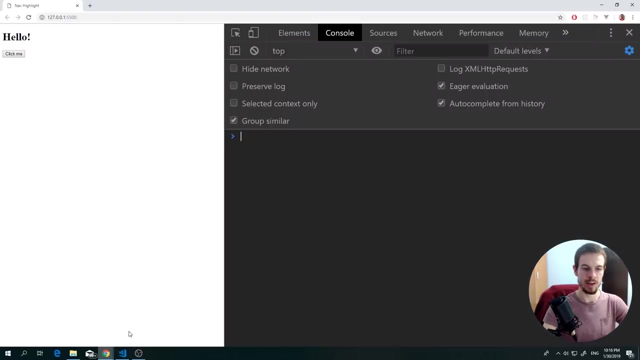 dot title And let's add it to the button as well. we're going to add a class of change color And in here we can const: change color is equal to document dot query selector. we're going to say change color like so Nice, So we got those elements. let's see what we have in our HTML. we can close. 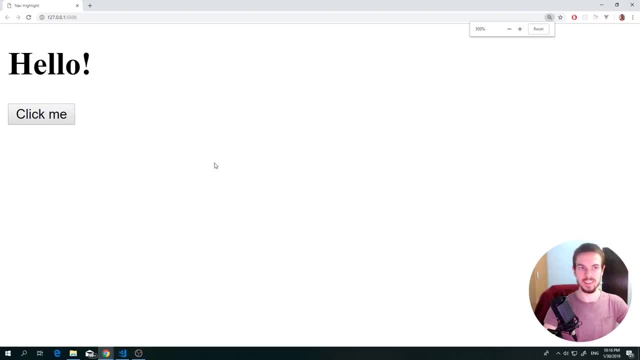 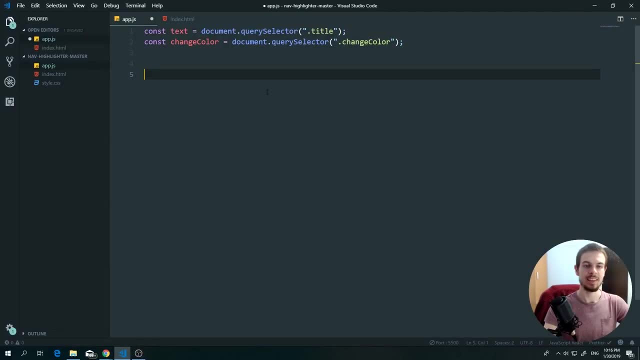 this, as you can see right there in the corner. I'm going to zoom this in like so- So we can see everything a bit more clearly And we can manipulate these any way we want. So we can do something like text dot, and there are a lot of different methods that we can use. So a popular 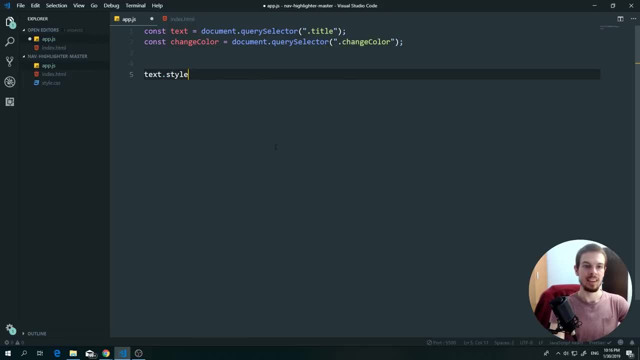 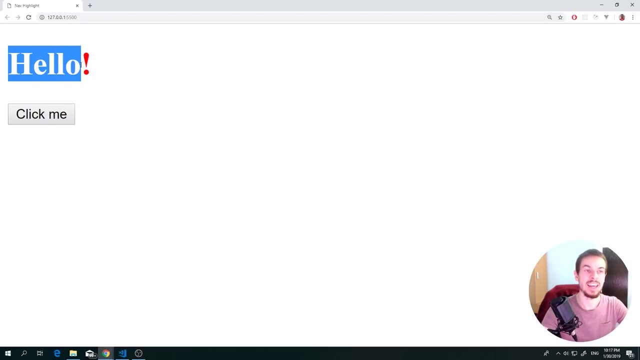 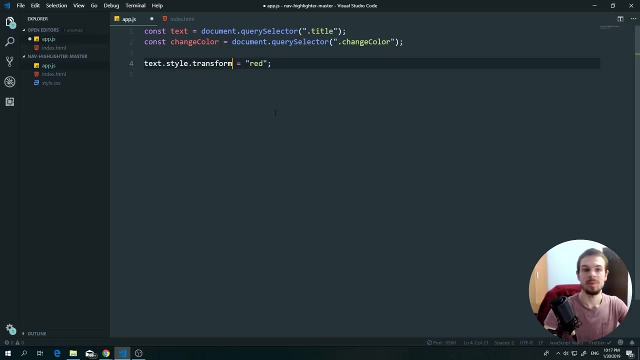 one that we can use something called style, And here, if you write dot, again, we can access everything that we have in CSS. So maybe color: if we set this equal to red, we can see that it's red. now, Nice, we can also access something called transform, And then we can translate this any way. 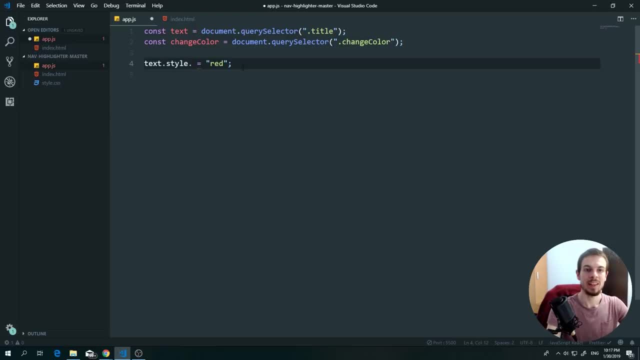 we want, And one thing to keep in note is there are a few of them like background color that is not going to work with the normal line, like so. So the only difference here is that we need to uppercase the color And then it's going to work just fine, like so: Ooh, that red is hurting my eyeballs, So we can do. 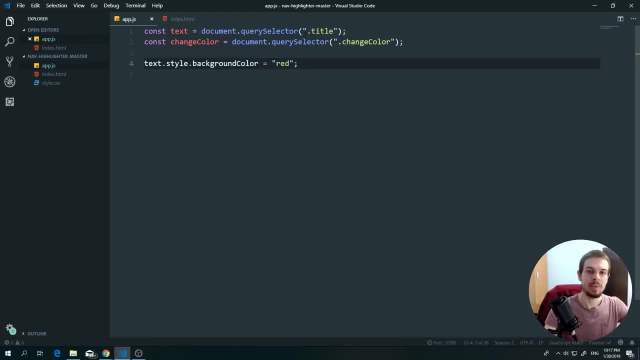 different things In our JavaScript. we can manipulate them. Another popular thing that we can do is add classes to them. So the way you can add classes, well, let's create one here And we're going to call this. let's say: 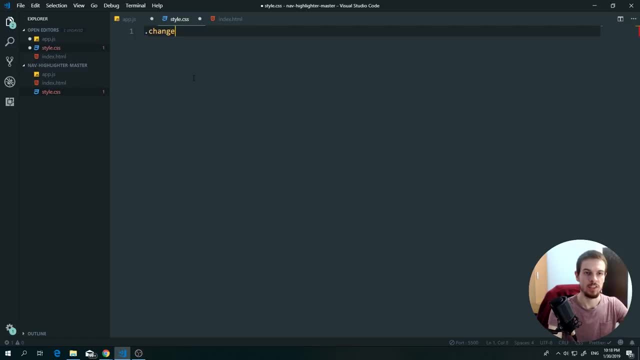 change, change color. the same thing we did so far. we're going to add color: light blue, And we're going to change the. let's just change the font size to 500 pixels as well. We're going to. we're just going to add, change, All right, and then we are going to add a border of 10 pixels, solid black. Okay, Now the way we can add classes is saying text dot, class list. This is going to access all the classes that the text has, And then we can do dot, add, And in here we can just say change. 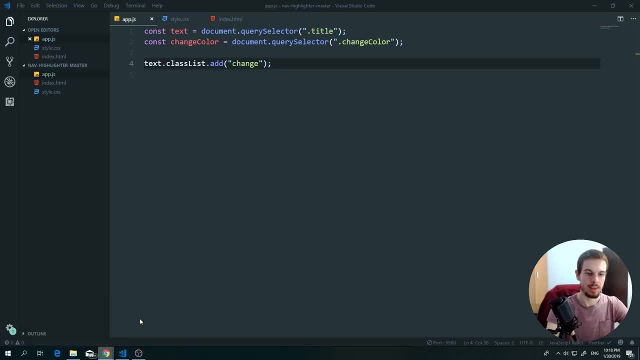 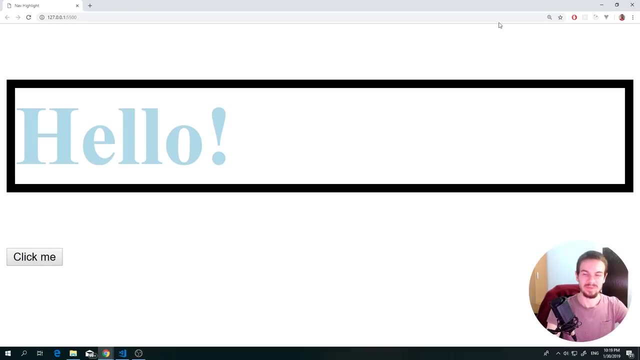 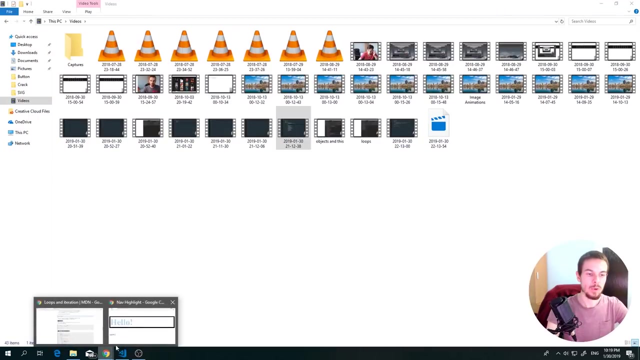 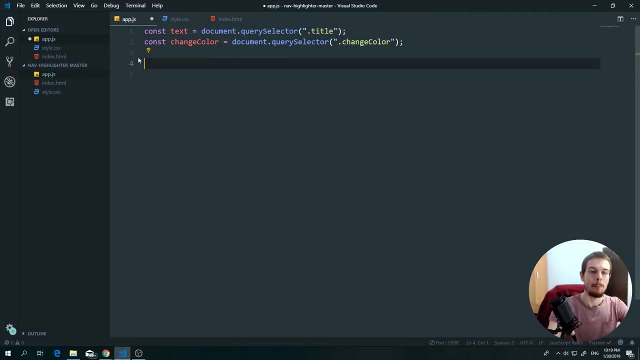 make some supposed to this beautiful looking class. Now we can also remove one, if we want, by adding, remove and we can toggle, which we are going to get into just a bit, And once we're done like this, obviously you can delete a lot of the revision that you want. 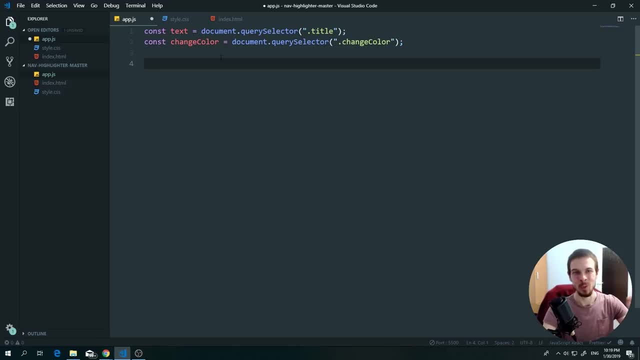 to do, but I will show you how to do that. So to do event listeners. So what an event listener is is basically a function that's going to execute depending on what the event is. So you can have a click event, you can have a scroll event. 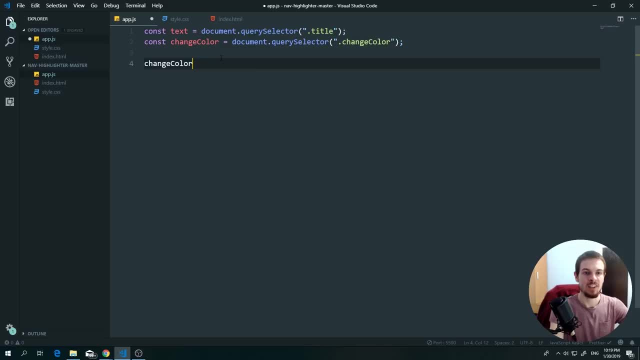 So maybe you can have the change color here. And if we add the event listener- and this is basically a function that's going to take two parameters- it's going to take the event And so a click. So if you want something to happen when you click on something, maybe when 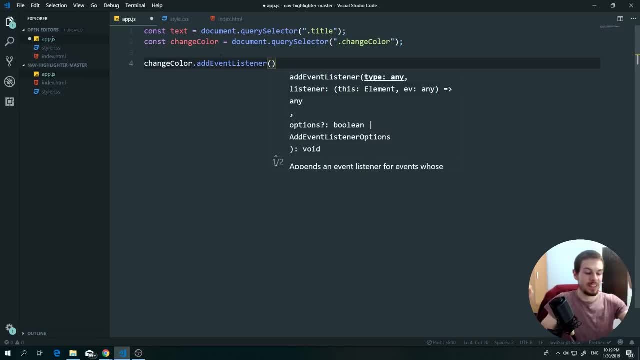 you scroll, maybe when you press your keyboard down, there are tons of events out there. I'm going to leave on in the description a bit of note on where you can find all different events that you can use. So let's cover one click in here And here we can just create a simple function. 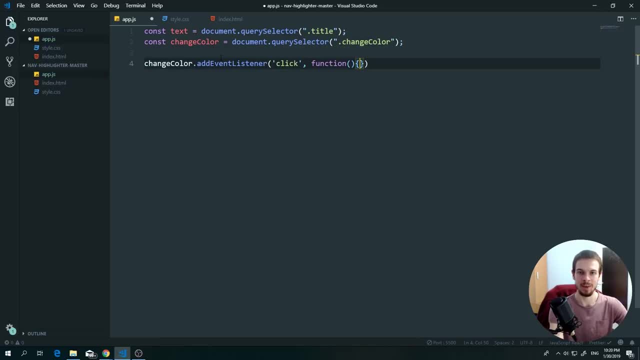 And like so. So again, let me go back a bit, because this can be a bit confusing. So just, we have the click here and we the second parameter is going to be the function. So what's going to happen here is: 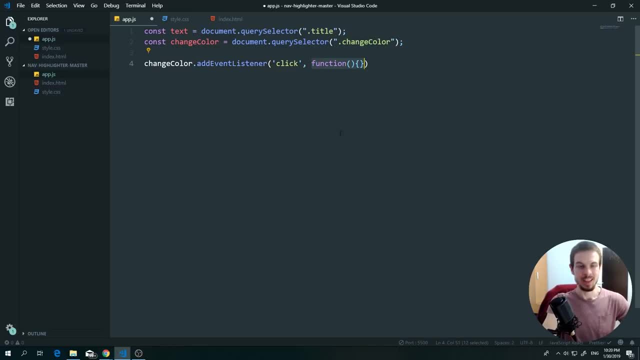 when we click, this function is going to be executed. So this function is not going to be executed when the page loads, only when we click, And this is something called a callback function. So after we click, the callback function gets executed. Okay, so in here. 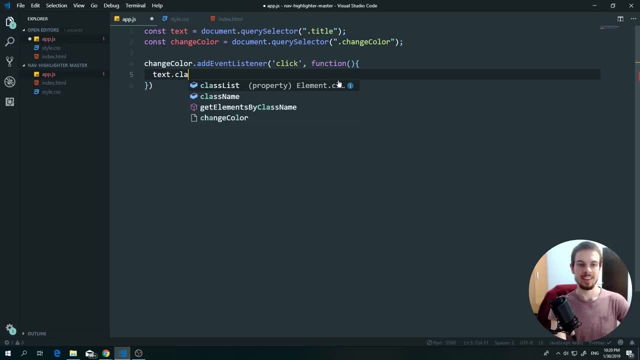 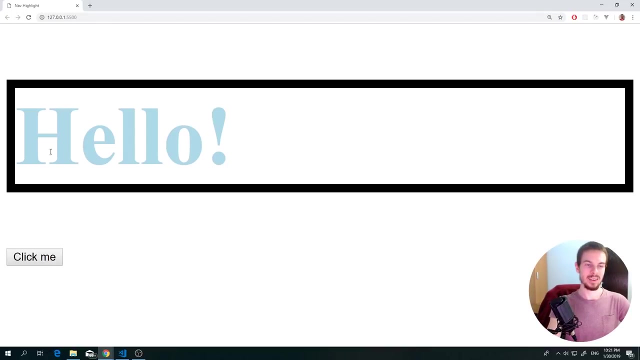 we can do something like textclasslistadd And we can do- I don't remember- change. There we go change. So if we hit save, we're going to see that when we click boom, the class gets added Now. 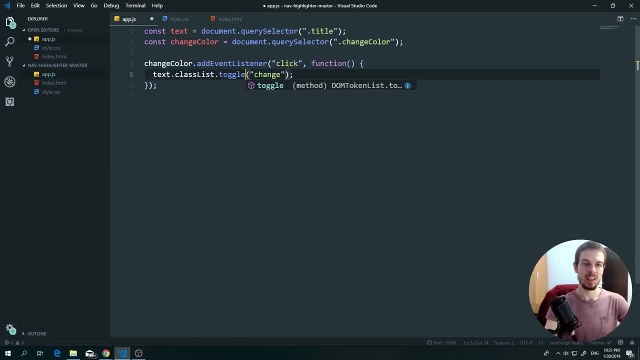 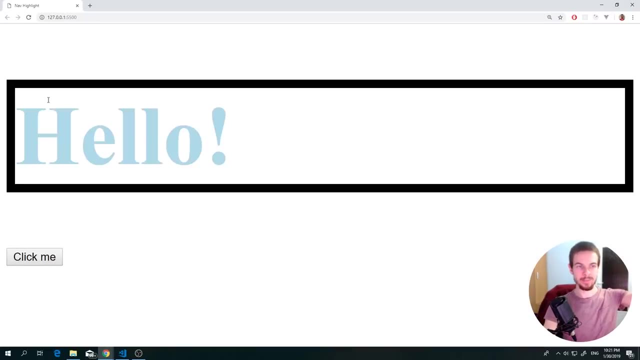 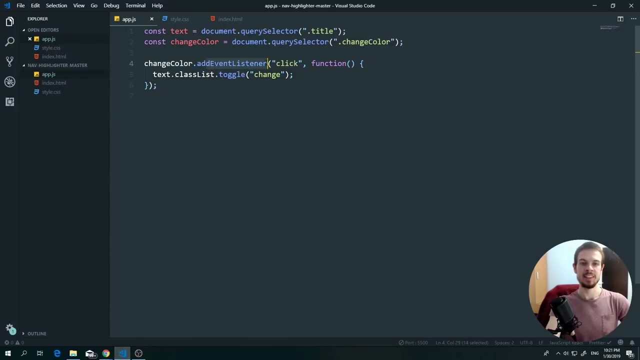 another cool thing we can do is add toggle here, So not add. we can add toggle Now if we click, and if we click again it's going to remove that class Like so Nice, So that's an event listener. Another cool thing that we can do is let's say we have 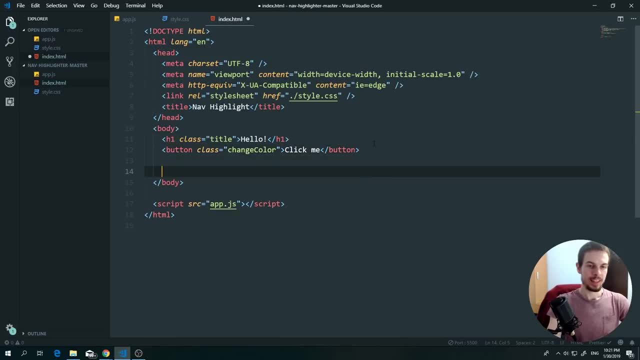 multiple texts in here. So let's say we have a nav And we have a ul And just have some li's- actually A ul with a couple of li's- Add, Copy, paste this multiple times. We're going to say John, Joe, boy and Harry. There we go. So 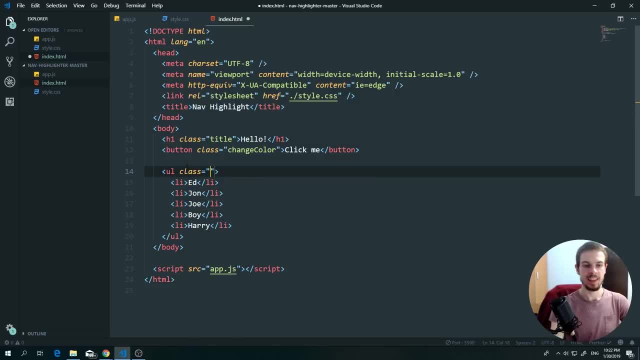 let's name this, add a class to the ul, And we are going to name this name list like. so Let's add the like this: okay, Name list. So we have a name list with the li's. So another thing. 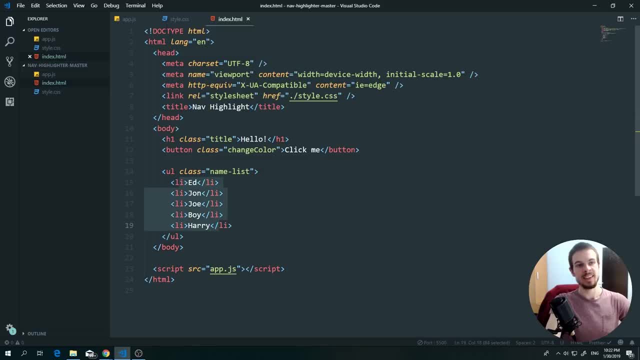 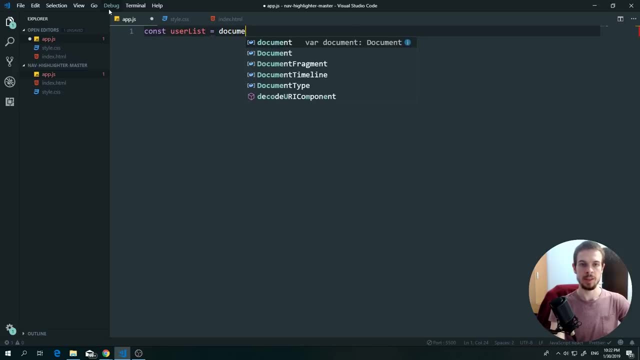 we can do is we can select all of the lists at the same time, And the way we can do that is we're going to say const userList is going to be equal to documentquerySelector And we're not going to be using the querySelector. We're going to be using the querySelector all because we want to get all. 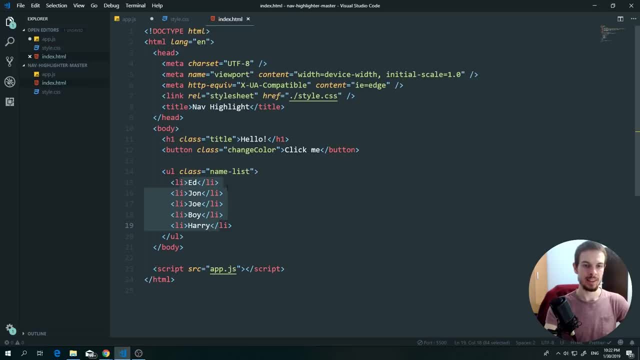 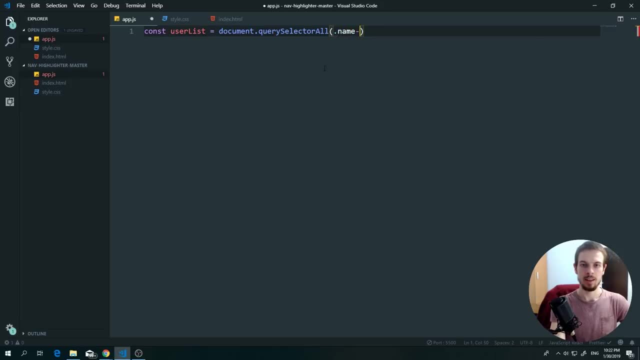 inside this ul. So the way we can do that is we can say name list li. So we're going to select the name list. class Name list. Oh, we need the quotes Dot, since this is a class Name list Li like. 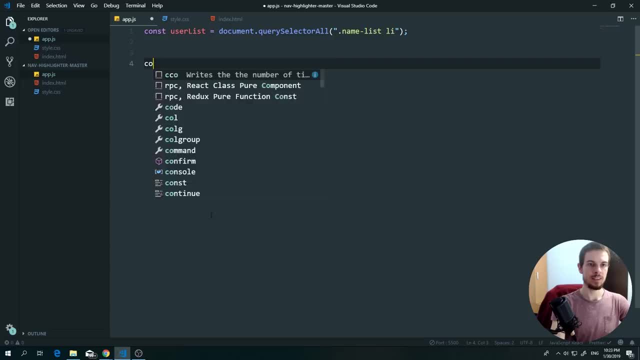 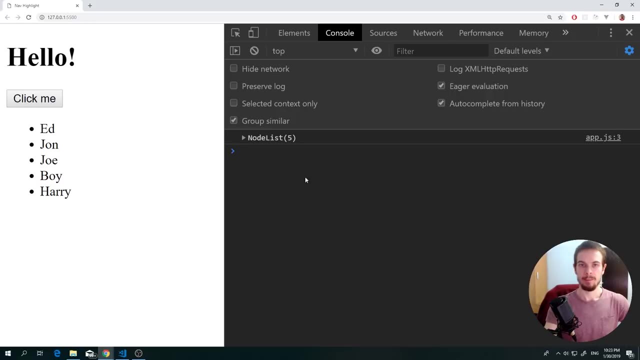 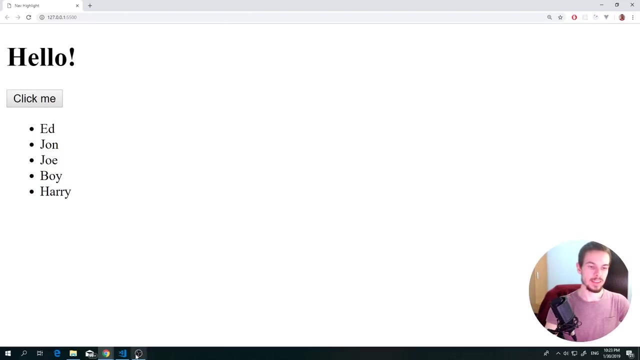 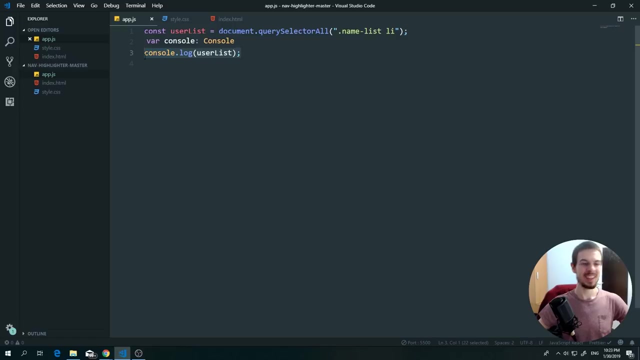 so This is going to return us if we console log userList, it's going to return us all the lists in here: Zero, one, two, three, four, as you can see. Good, Nice. So we can also take these and manipulate them the way we want. And remember, in the last video we used loops. 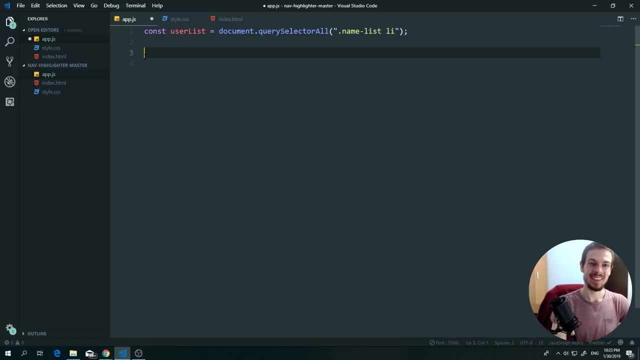 So hey, we can use loops again And a cool way we can do them is say, for we can say user of userList, okay, And here we can access each individual user and do something to it And we can get the user, so each individual list, And we can add an event listener. 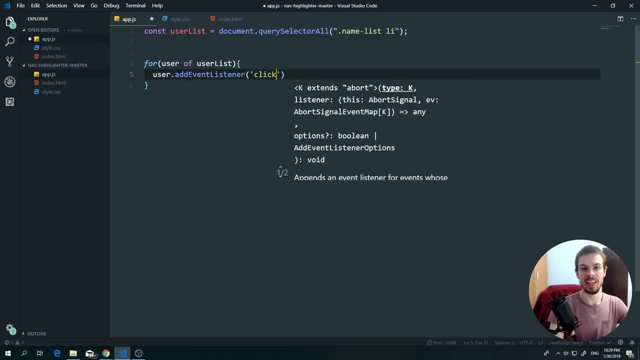 to each. And then let's say we want to listen on a click And here we can run a function And, if you remember, in my previous video we can use the keyword this, which will mean the element that we're going to click on. So this in this context: console log. 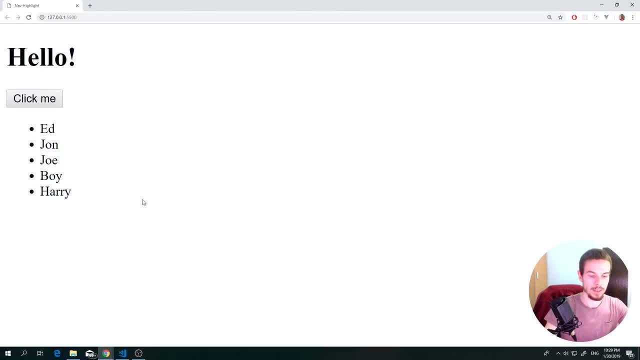 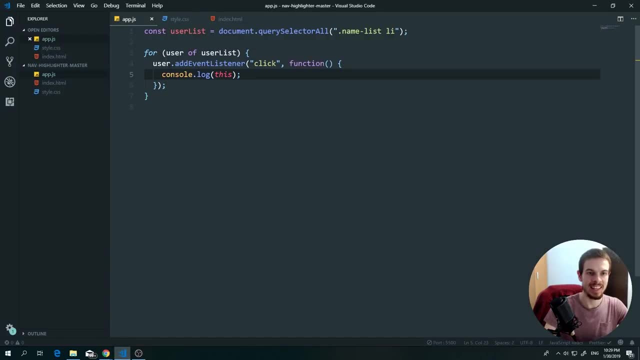 this is going to be each list: Click, click, click, as you can see. So again, just look at the left and you're going to see what this is. So what we can do is also do something like this: dot style, dot color: It's going to be equal to red, And now, every time we click on this, 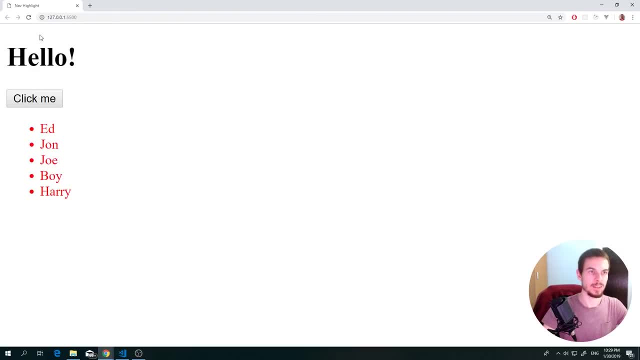 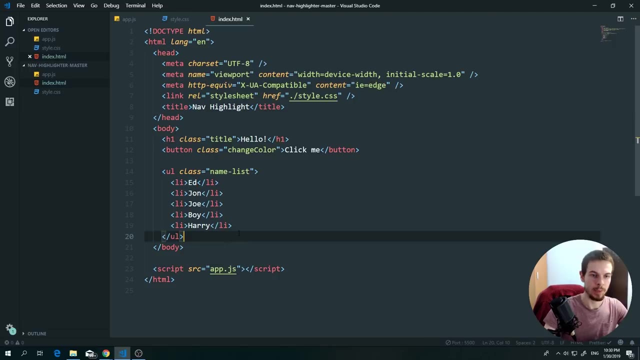 it's going to change its color, So that's pretty cool. Maybe you can do something like you have a button on each, And every time you click you can delete or you can add. We can also use something called let's do add an input in here. So below our 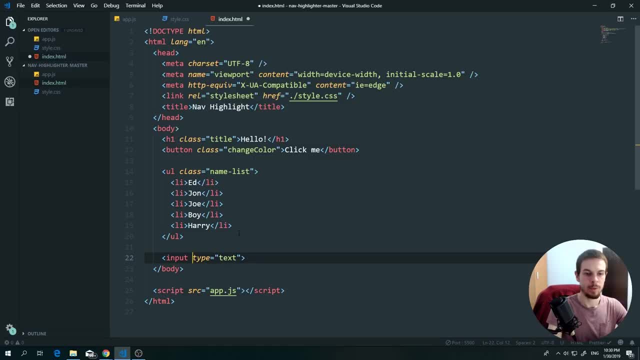 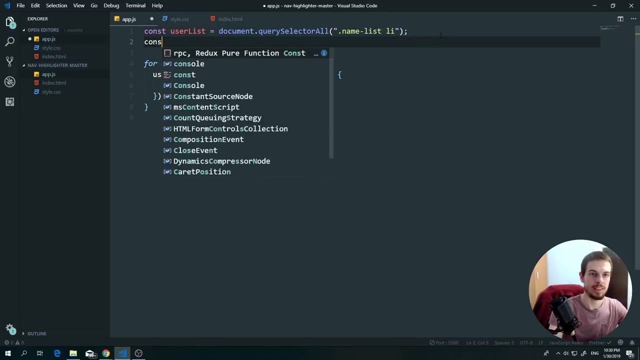 ul. we can add an input type text. We're going to add a class of. let's add a list input. We can get it, So we can add it in here by calling const list input. I'm going to camel case it. here We're. 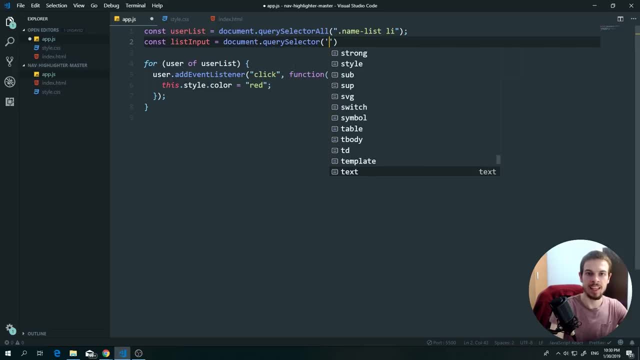 going to say document dot query selector and we're going to get the list input like so, And the way we can get the value is by list input: dot value- Cool. So let's delete this and modify a few things, All right? 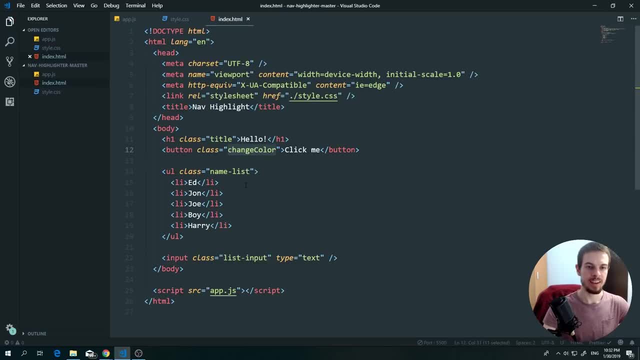 There we go, go. We're going to delete this as well. And here let's say we want to change the functionality of this button. it's going to add a list, add list button like so: Copy this. we're going to go back. 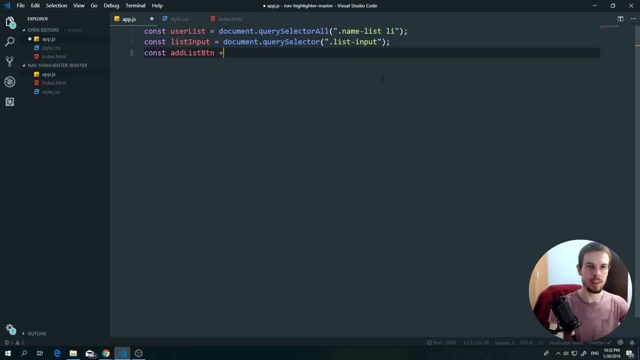 here we're going to say add list button is going to be equal to document dot query selector And we're going to add list button like so. So add list button. we can add an event listener to this And on click we want to run a function. So what we can do here is we can create an element, So we 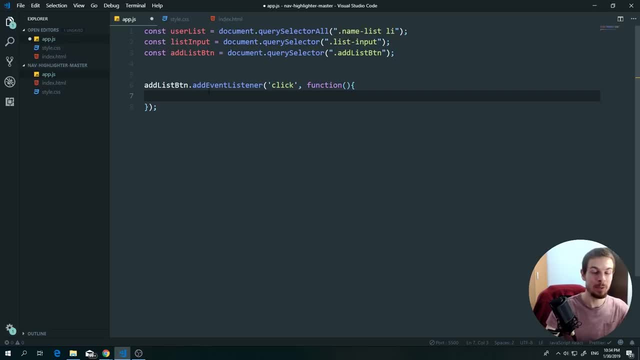 can create an ally. we can add the value of the input inside that ally and then we can attach it to our list. So there are three things that we need to do here: create an ally out of tin air- here we need to. 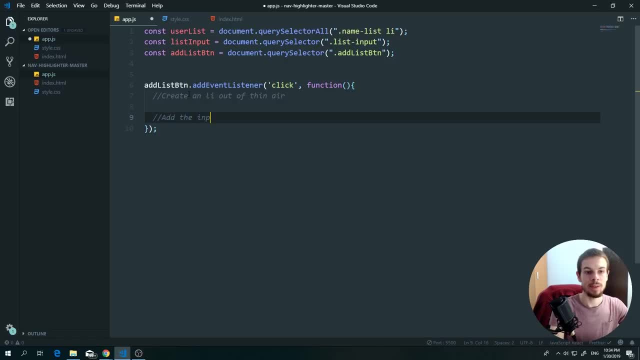 add the input value inside that new ally that we created, And then we need to basically add the ally to the user list in here, So attaching the ally to the user list, Okay. so let's do these three, Okay. so there's one thing I modified before we get into this. I removed document dot. 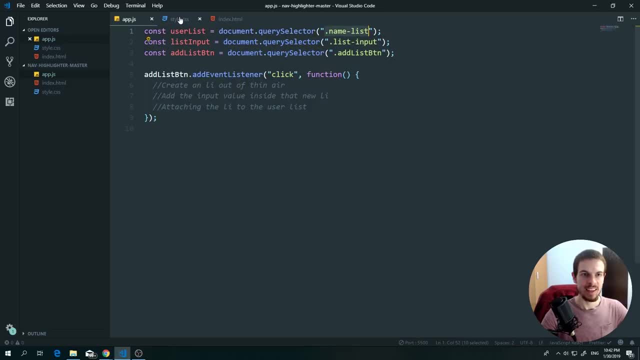 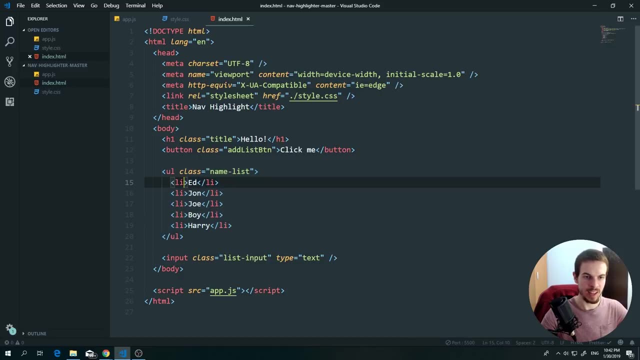 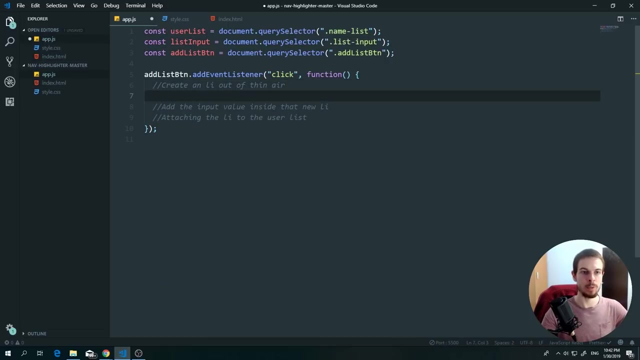 query selector, all, and I just added name list. So right now all we're doing is we're console logging and we're just getting the UL- Okay. so we're not getting each individual list, we're getting the whole UL, Okay. so how do we do this? so we need to create an ally out of tin air, I know. 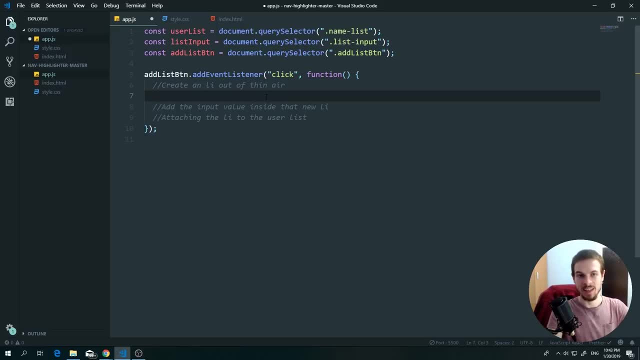 that sounds magical, but it's way simpler than you might think. So we're going to write the cost called new ally And we're going to set this equal to dot query selector all, and we're going to set this equal to dot query selector all, and I just added name list. So right now, all we're doing is we're. going to create an ally and then I can just add name and we're going to provide the value that the base value should be, and then add button, So again we can create an ally. Now we're done, So we'll create a license. we've already created license. we're done, So I'm going to create an ami. 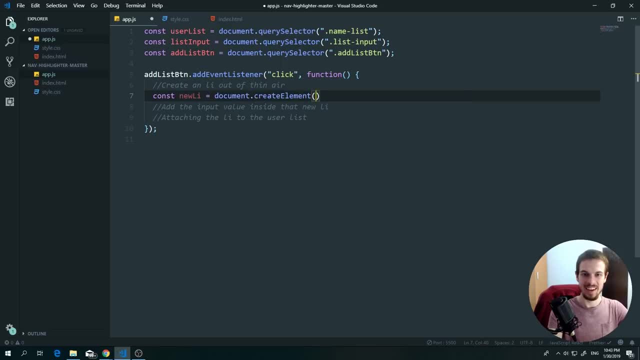 element, and here we have access to something called create elements. How nice. And here we can create a button, we can create an ally, we can create whatever we want. In this case, I'm going to create an ally, then uppercase all like so, And what we can also create is some content. okay, So we're going to create an ally. I, using the 49 Corona compliance suits using container database, container formt Pepper, know that there's no directory for free remaining account empty for this document. Okay, so I'm going to take the new item you just took out in the builder and add a new item. 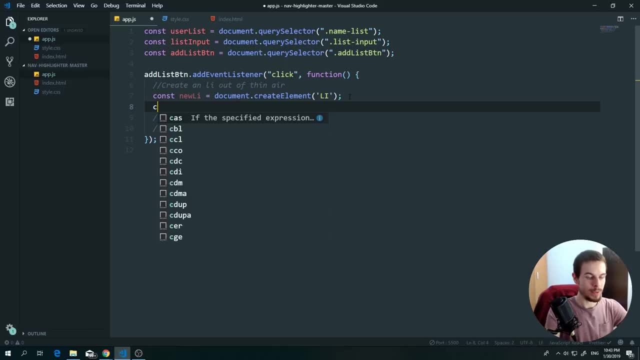 that we can insert into this li. And the way we do that is we're going to write const And we're going to say li, content is going to be equal to- and I'm going to say document, dot. create text node. Okay, And here, rather than passing something random, we want to dynamically add: 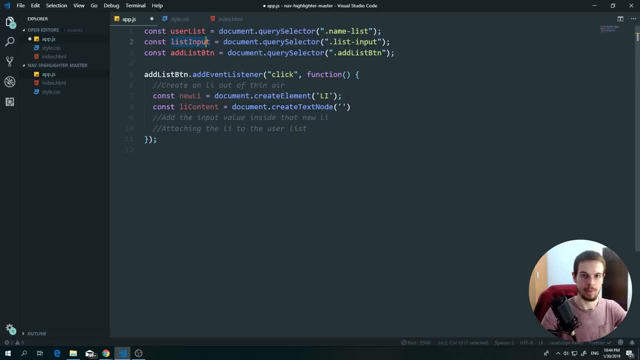 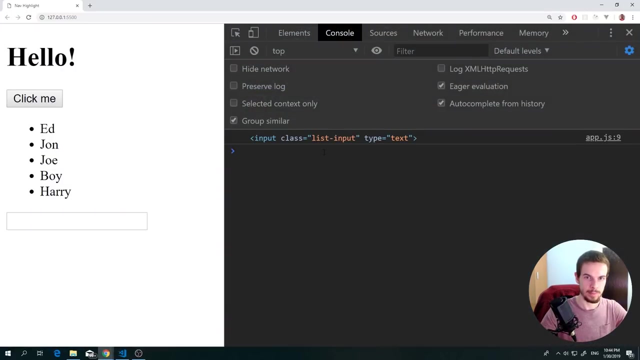 whatever we get from the input. So remember we can get the value of that input. Let me just add something random in here. But if I console log list input, we are going to get the input Like so. And if we do dot value, we are going to get the value Nothing. There we go. 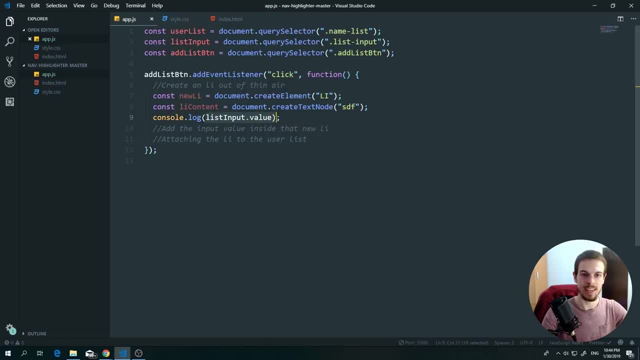 So, so, so. so what we can do is we can dynamically add this in here like: so Good, Now what we need to do is attach this content to the li. So let's do that. The way we do that is, we write new li. 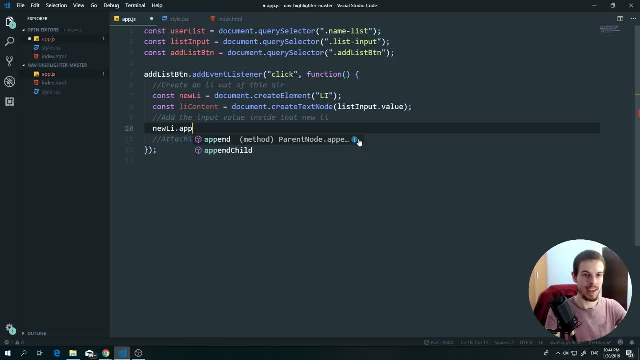 dot append child And we can add the li content in here. Good, So we attached, we appended the content to the list And now we need to append the list to the user list Inception all over again. Okay so, user list, dot append child And then we can do new li. Let's see.